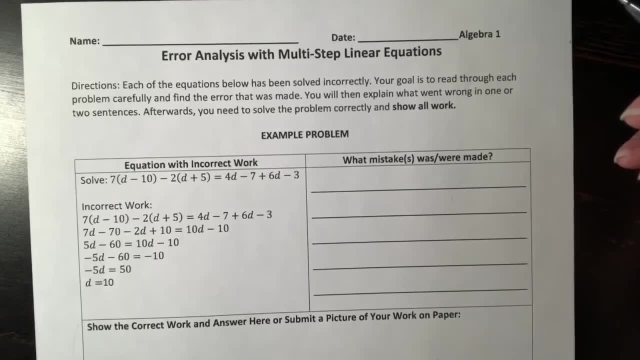 Hey everyone, this is Mrs Anderton here to give you a video of how to approach error analysis problems. You've been given this review activity to kind of help you get ready for error analysis, which you see a lot in SATs. Also, it's a good practice for solving multi-step linear equations. 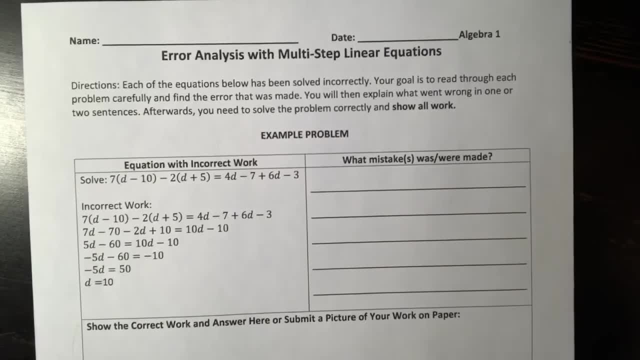 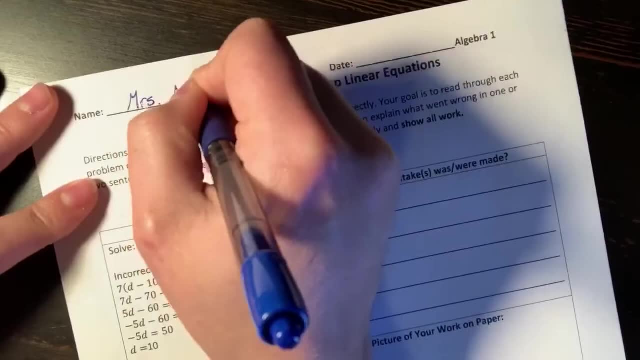 So the first things first. if you actually printed off this assignment at home, you can simply write your name at the top. It's always a good idea to do so. So I'll do that real quick. And there we go, And the date's kind of optional, given everything. 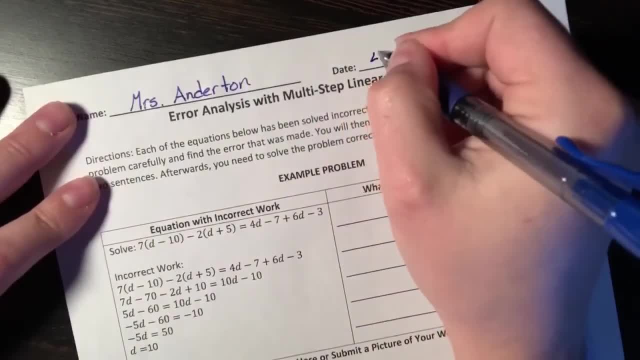 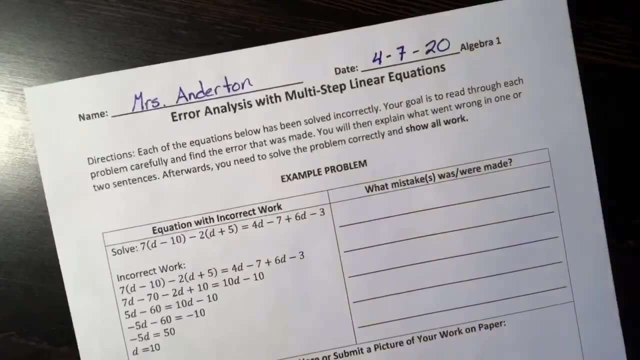 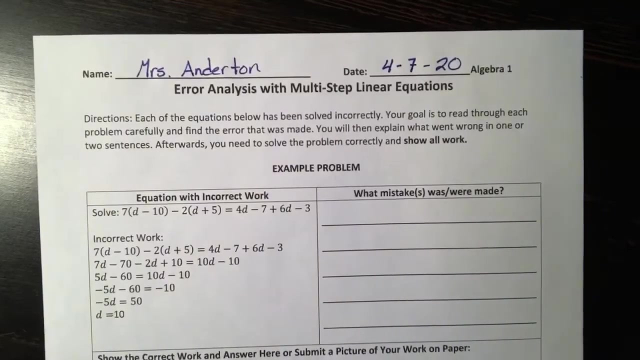 that's going on. I do know that the days tend to run together, but for me today is April 7th 2020.. And what a year it has been All right. so we got this assignment here called error analysis, with multi-step linear equations. So the directions say each of the equations below: 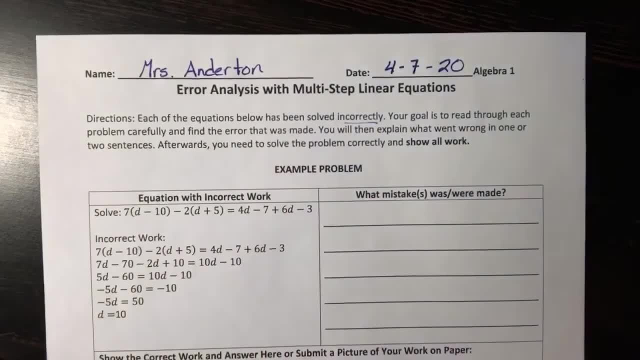 has been solved incorrectly. Okay, Your goal is to read through each problem carefully and find the error that was made. You will then explain what went wrong in one or two sentences Afterwards. you need to solve the problem correctly and show all work And you'll notice. that is in bold because we do want to see. 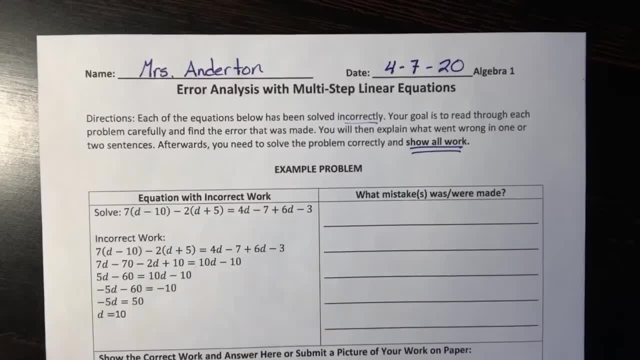 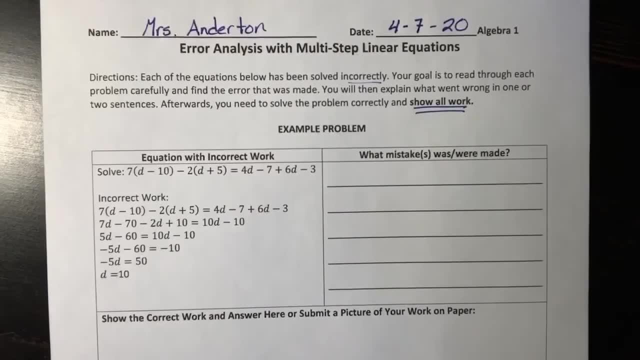 all the steps you did. The first problem: this is not part of your assignment. This is actually just an example problem to give you an idea of how this works. So you're going to have to do a lot of work, You'll notice. on the left, here's the equation with the incorrect work. So this is the 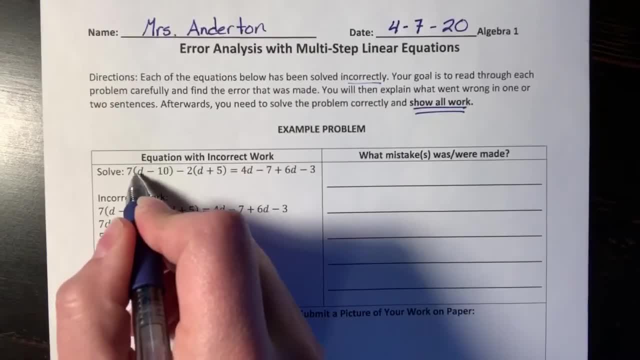 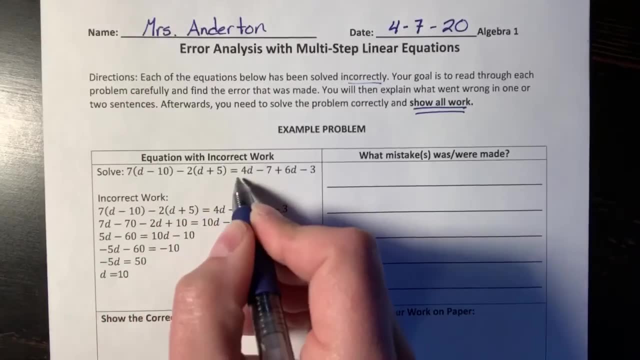 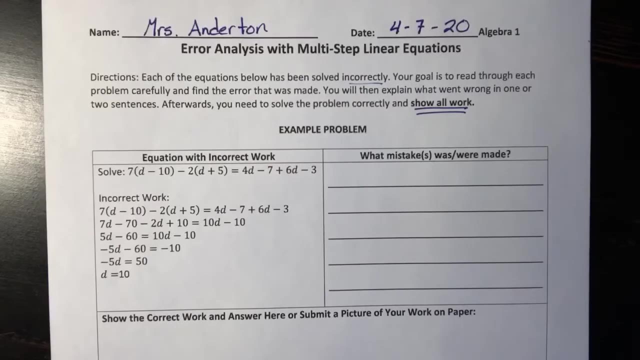 original question. It says: solve seven parentheses D minus 10 and parentheses minus two. parentheses D plus five and parentheses equals 40 minus seven plus 60 equals three. Now some of you might be staring at this problem saying that's a big one. Well, keep in mind, this is an example problem. 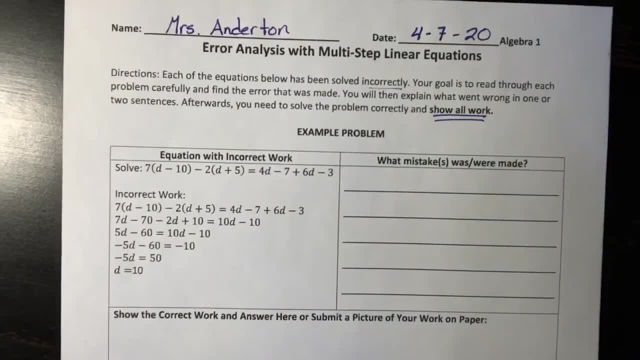 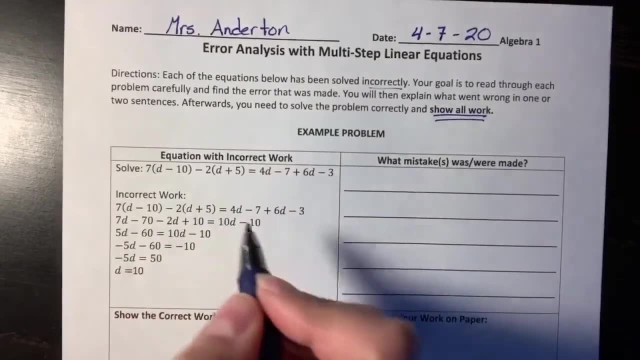 The goal here is: I want to give you one that is longer, So that way you don't have to do it on your own later. Okay, So here's the incorrect work, And we're just going to kind of read through it real quick, See if we can spot the error. Okay So. 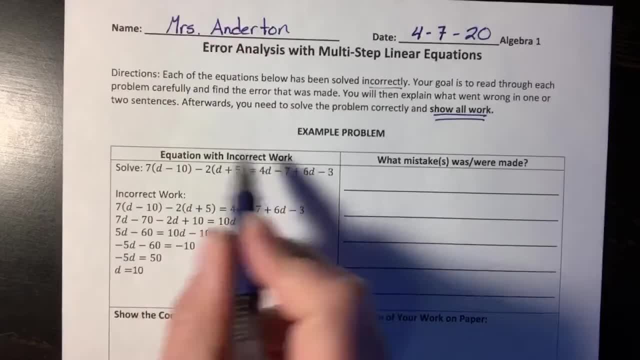 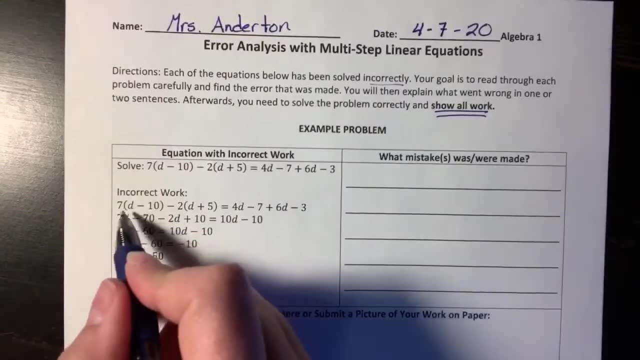 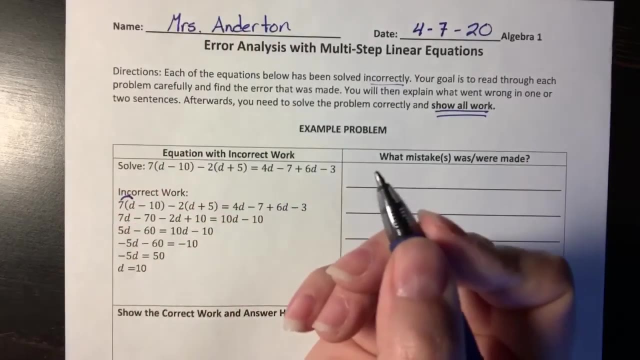 the first line is just a copy of the original problem. It's always a good idea to write down whatever problem you're starting to solve, Okay, And then it looks like if we've got parentheses, they did some distribution. So you do seven times D, which is seven D, And that looks good. 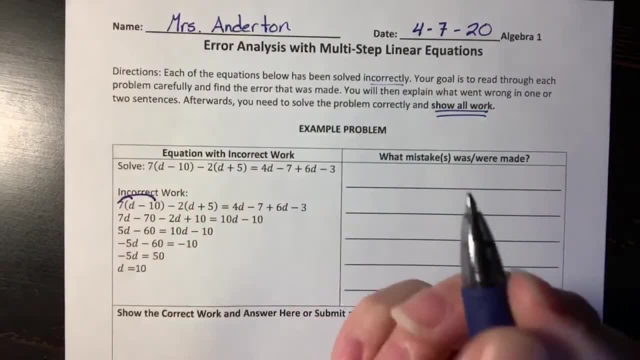 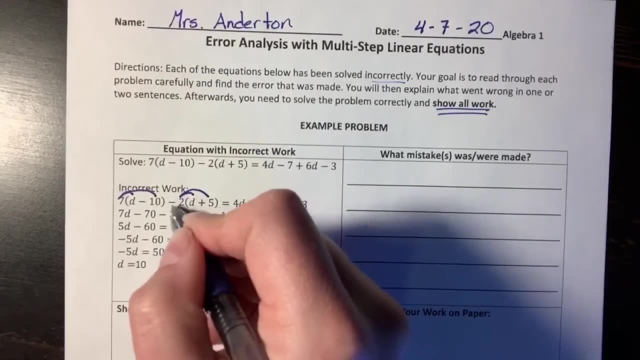 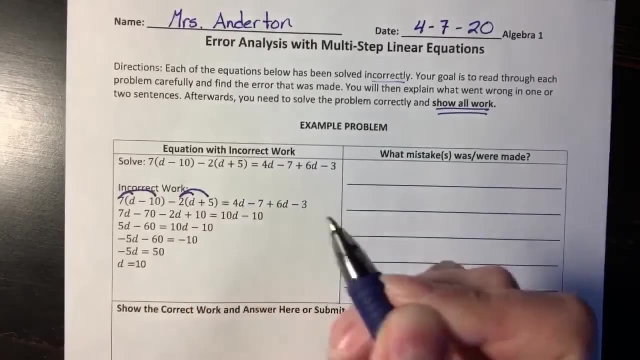 Seven times negative 10 should be negative 70. So all good there, And then we're going to have more distribution because, again, if you see anything, any number, in a set before a set of parentheses, you're going to be multiplying that number by everything inside, And so we are going to do negative two. 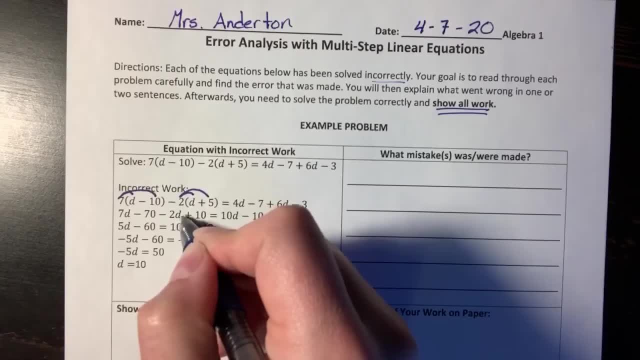 times D, which is negative two D, So that looks good, And then negative two times five. Oh, I think that's our error. here We have a positive 10.. And those of you that remember, if you multiply a negative times a positive, the result- 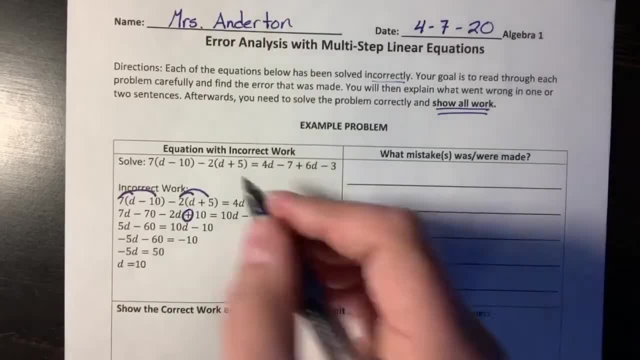 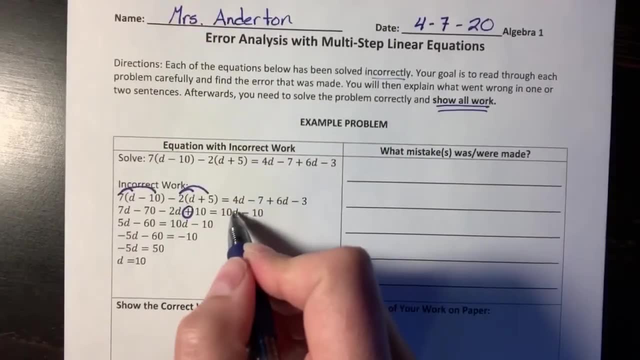 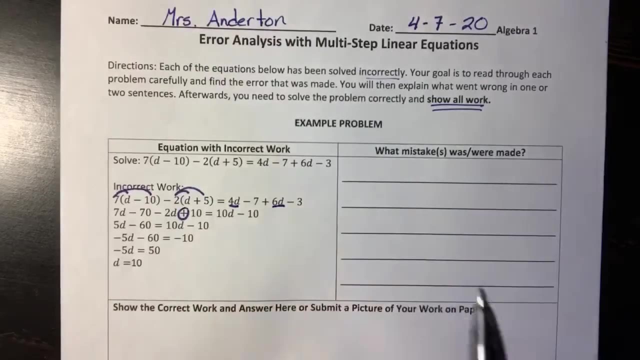 the product should be a negative number. So that is definitely an error there. And then just kind of continuing on, just to see it looks like on the right side of the equal sign they just combine some like terms. So I see a four D and a positive six D. So together those do combine to make 10 D. 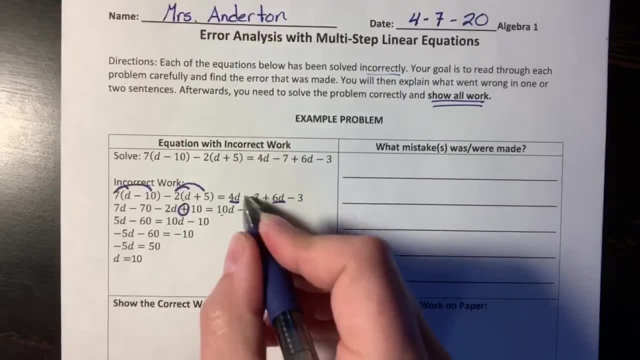 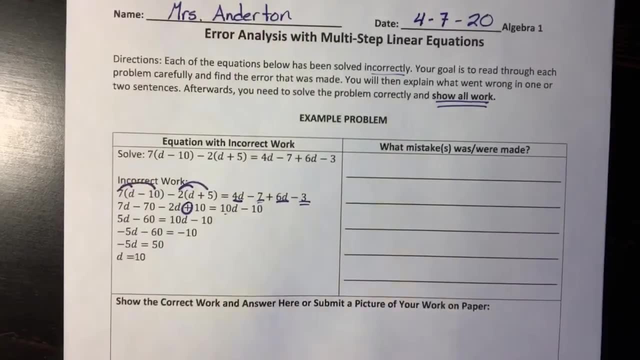 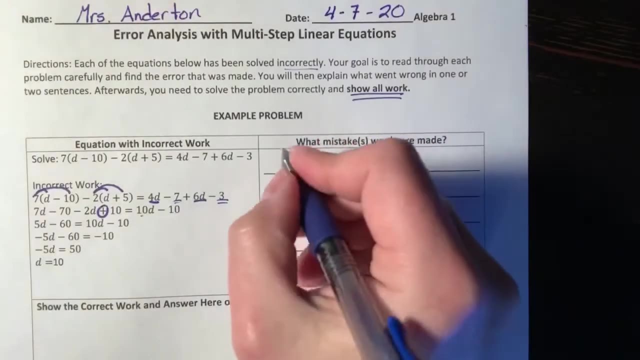 That's all right. And then we've got negative seven and a negative three. Those are also like terms. So negative seven minus three should be negative 10.. So all good is good there, but that's definitely a mistake. So what mistakes were made? Well, you may want to go ahead and write now, right now that there 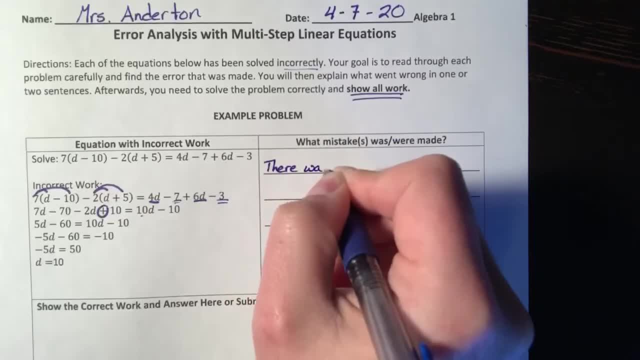 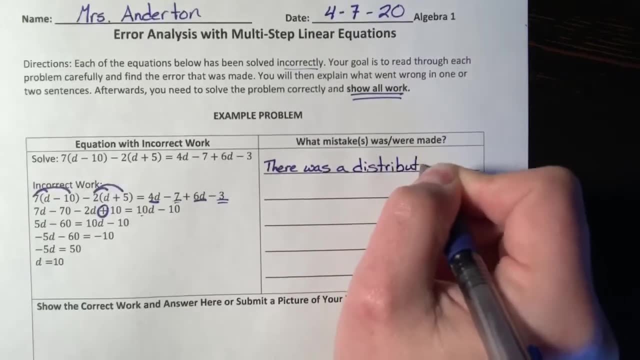 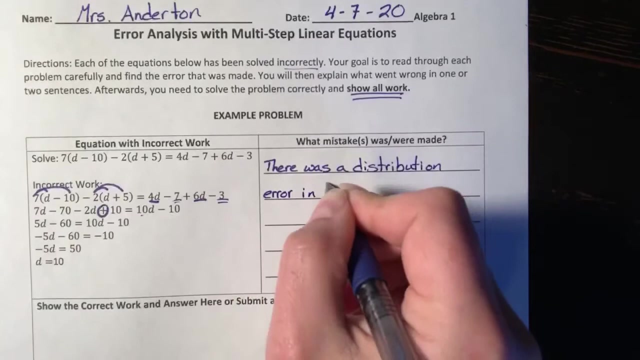 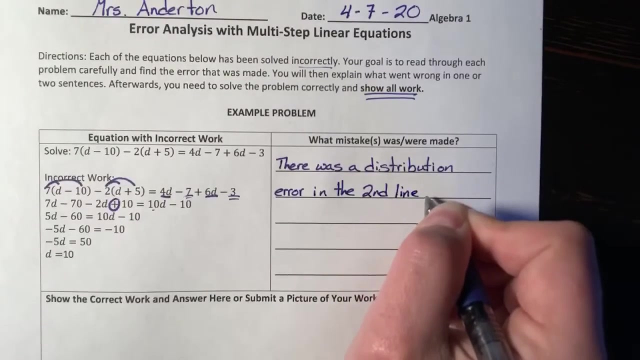 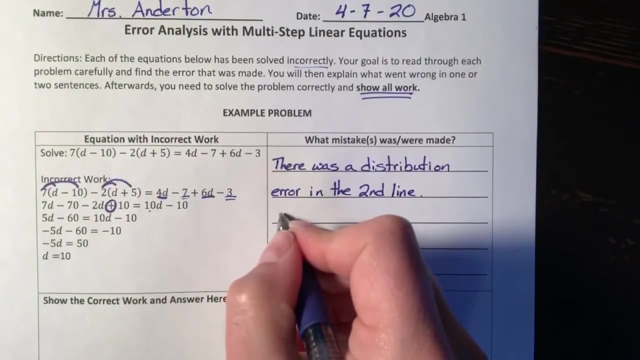 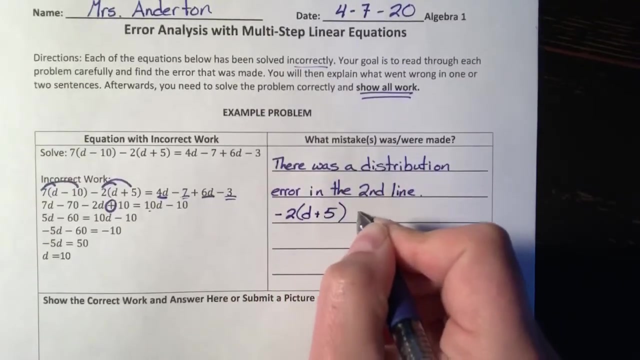 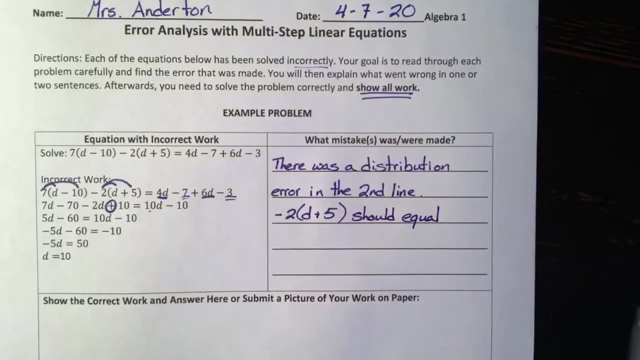 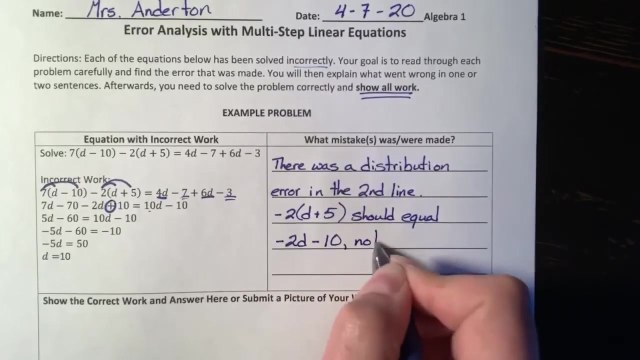 was a distribution Error In the second line, And then we do want to include some details about what the error was specifically. So I'm going to write out that negative two parentheses D plus five Should Equal D, And I'm going to say negative two D minus 10, not negative two D plus 10.. Okay, So there's some. 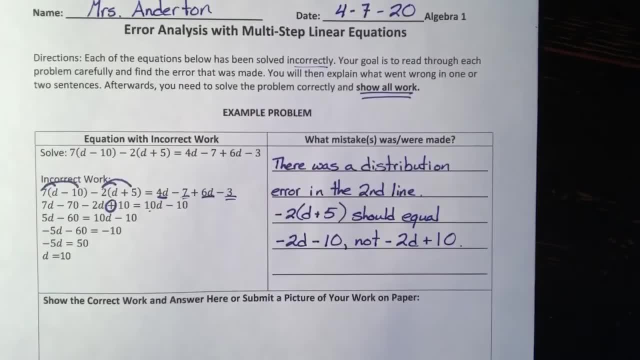 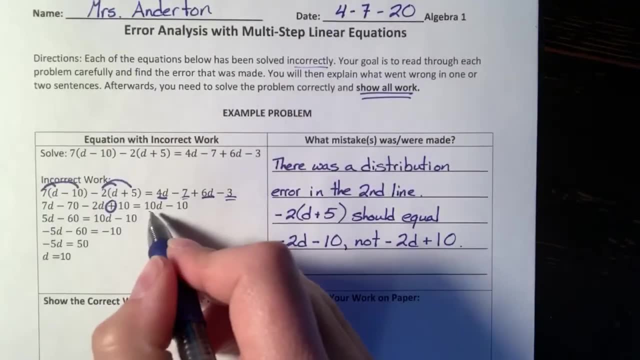 details about what the mistake was that was made. I'm just going to keep going through. There's actually going to be two errors in this problem, So I'm going to keep going here. So we ended up. this line was okay, And then kind of rolling with what they wrote. 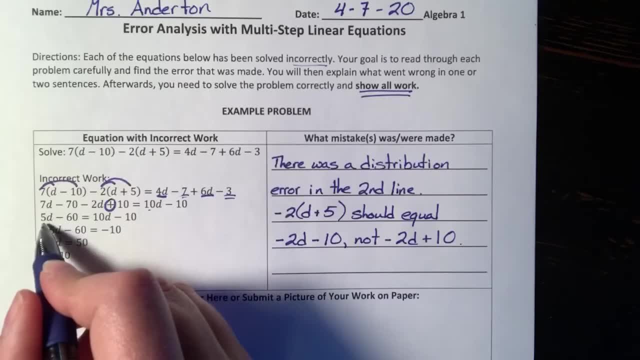 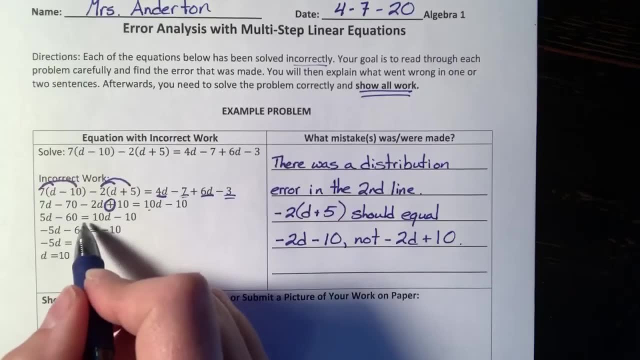 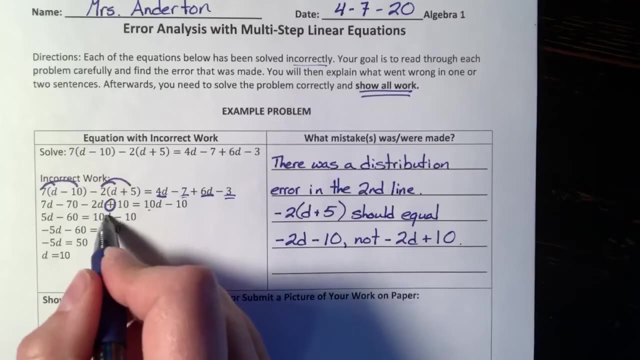 70 minus two D does make five D Negative. 70 plus 10,- even though that's not supposed to be like that- is negative. 60. Equals negative 10 D minus 10.. That's just the same. And then it looks like we moved the 10 D to the left side by subtraction. So if we do, 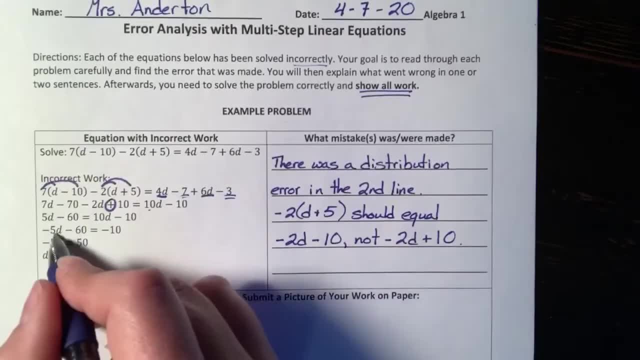 Minus 10 D, minus 10 D, we do end up with negative five D. So that's okay Then we do. We keep the negative 60,. keep the negative 10.. Down here, If I were to move this over to the right side of the equation because, remember, the goal is to try to get D by itself. 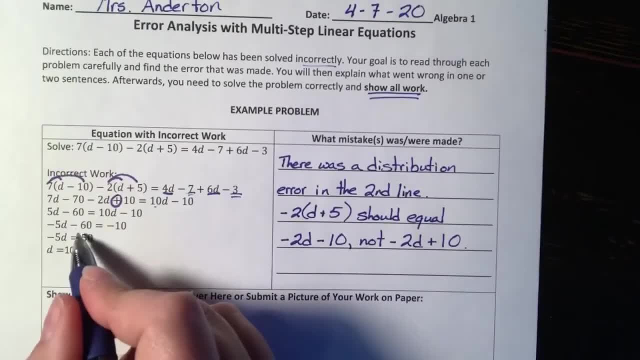 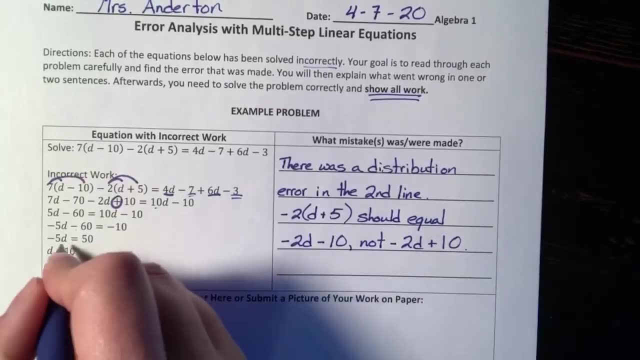 You would add 60 to both sides, And so it looks like negative 10 plus 60 should be positive 50. And then one last thing is, though, if we have negative five, D equals 50.. Here's where the error. second error is. 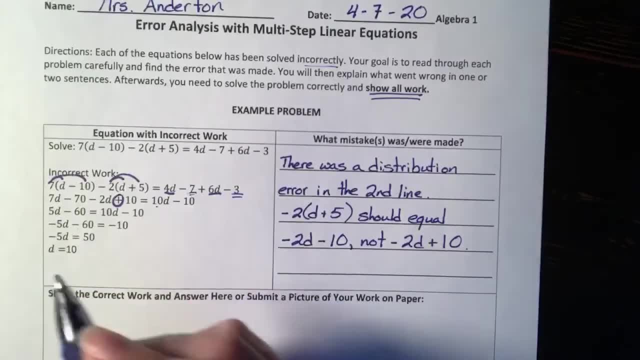 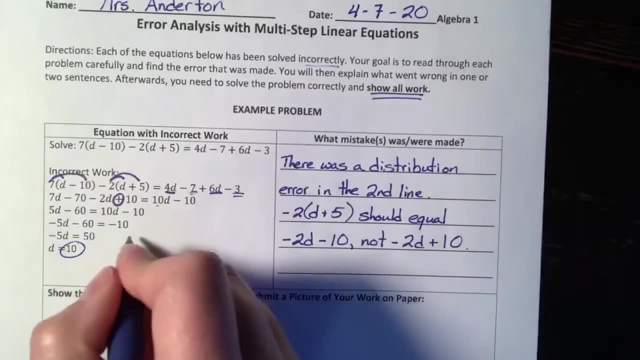 If I see negative five, D equals 50. I should be dividing both sides by negative five, And that should not be a positive 10. That should actually be a negative 10.. Now, that's still not the correct answer because of the earlier mistake before. 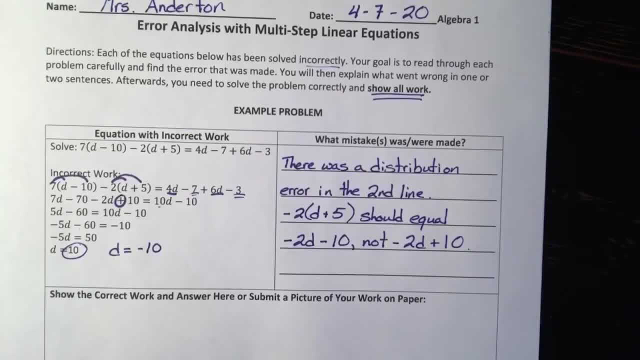 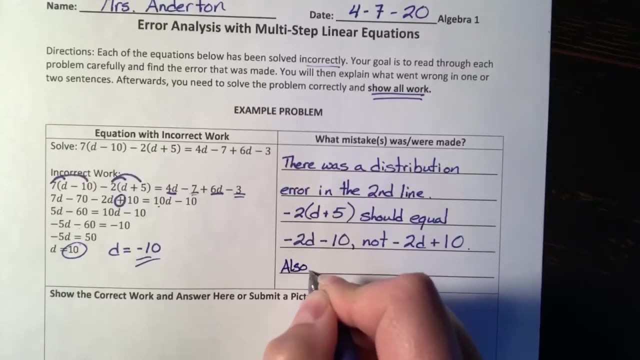 But sometimes it's nice to see if you can find more than one mistake in the math. Okay, Just a little reminder that when you're dividing a positive by a negative, your answer should be negative. Okay, Also, I'm going to add this as another mistake. 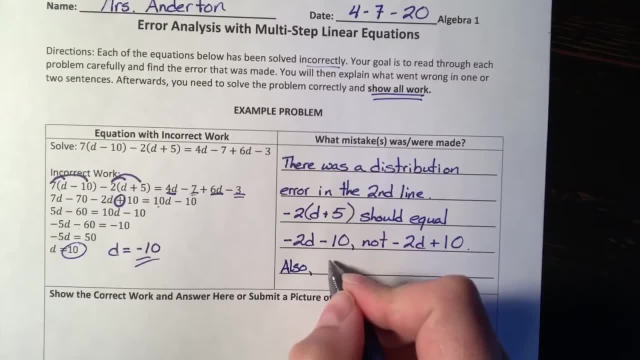 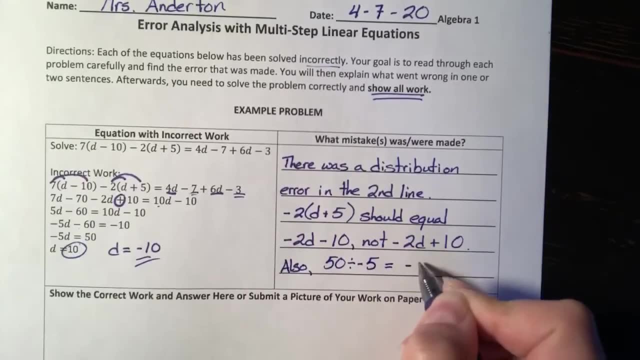 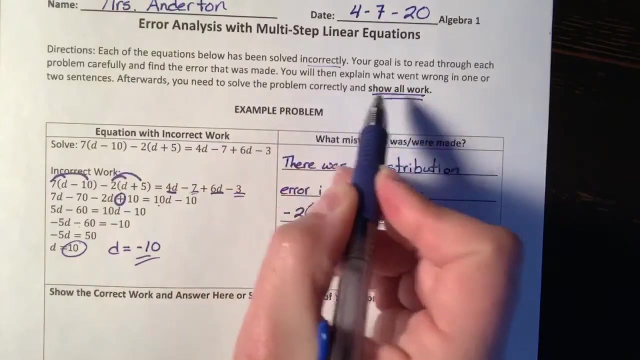 Also Negative, or 50 divided by negative five equals negative 10, not positive 10.. So there's another mistake that we found in this problem. So now the question is okay. It says afterwards in our directions: afterwards: You need to solve the problem correctly. 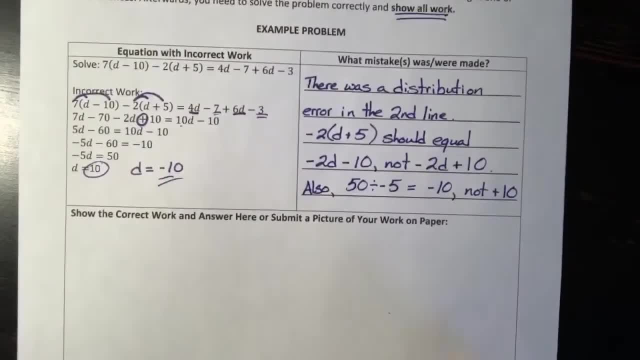 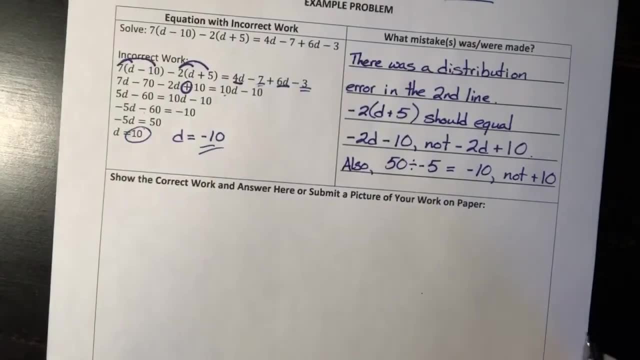 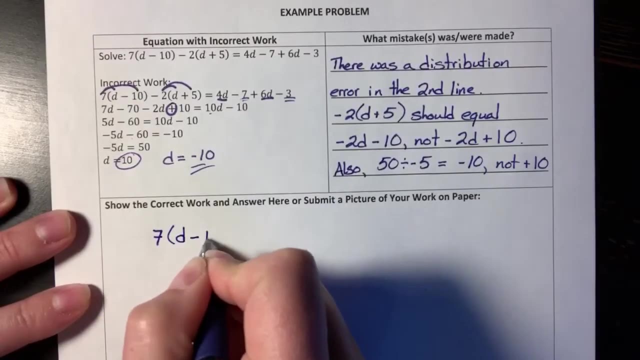 And show all work. So let's go ahead and show the correct work that should have been done in this problem, And you should start off by writing out what the original problem was. So I have. originally we had seven parentheses, D minus 10.. 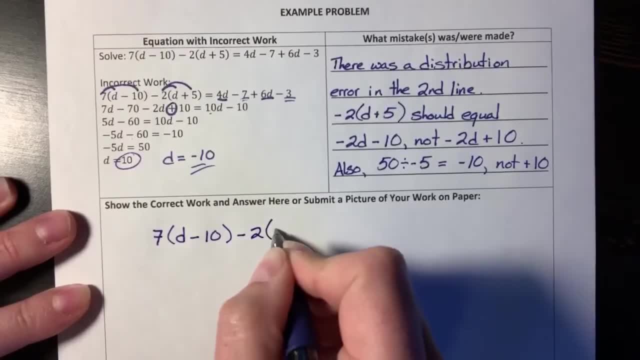 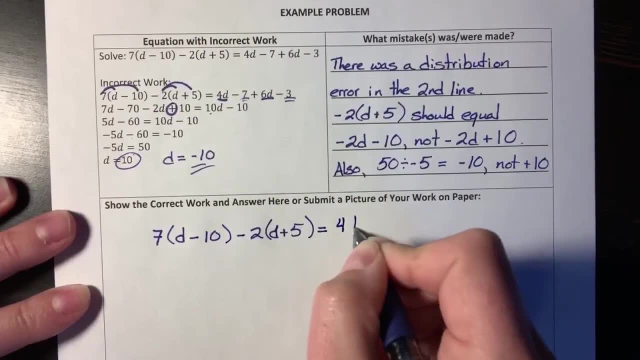 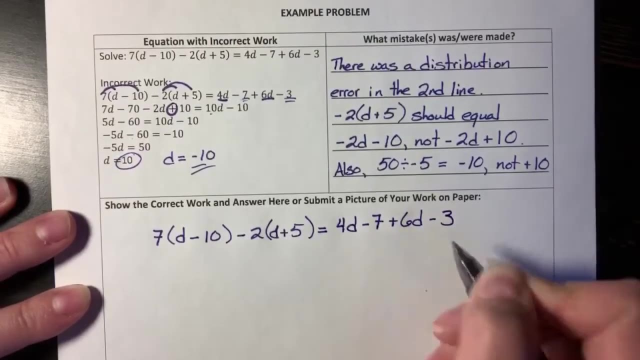 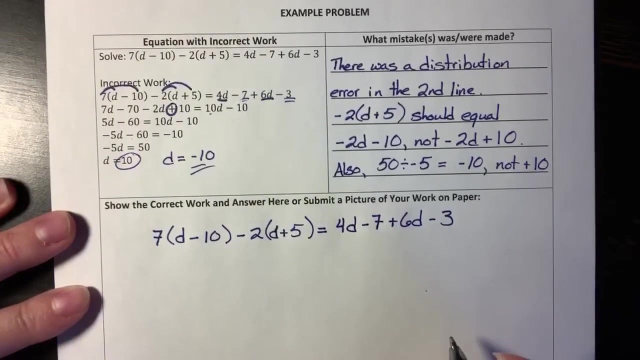 Minus two, parentheses D plus five Equals four. D Minus seven plus six D minus three. Okay, So there is the original problem. We're going to go ahead and work to solve this. So let's remember some of our algebra skills. 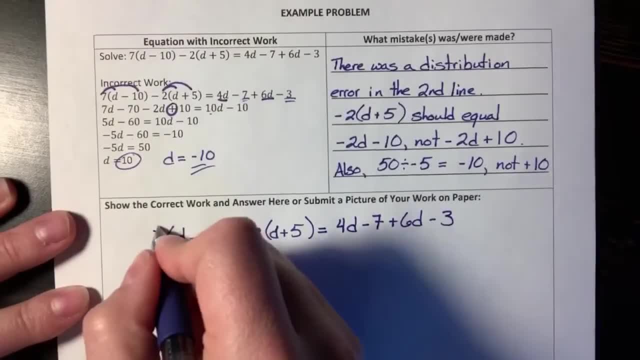 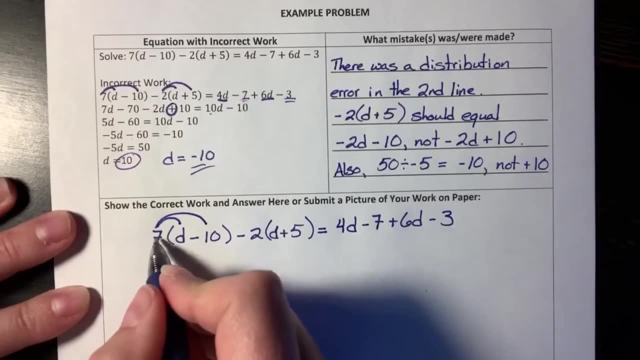 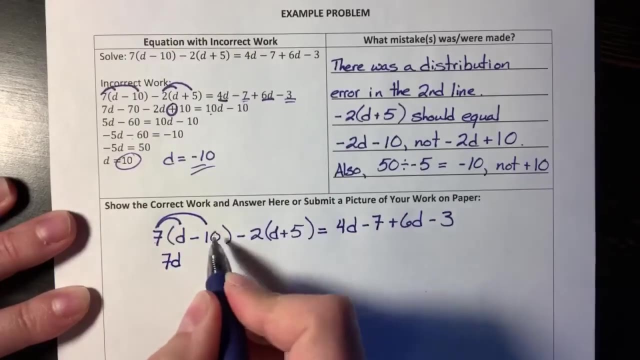 When we see parentheses and a number in front, we should go ahead and distribute. So I'm going to distribute the seven to the D and the negative 10.. So seven times D is seven D. Seven times negative: 10. Positive times negative makes negative. 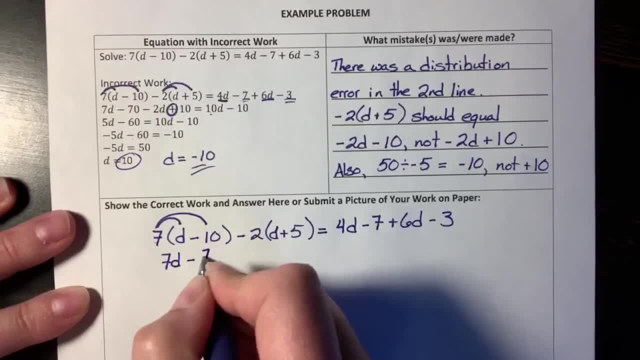 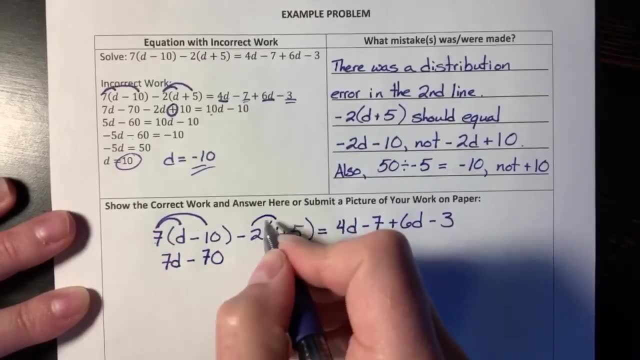 Seven times 10.. If you don't know that, use a calculator Is 70. Then it looks like I have another set of parentheses to deal with, So I'm going to do distribution again. Negative two: Remember to keep that minus sign with the two when you multiply. 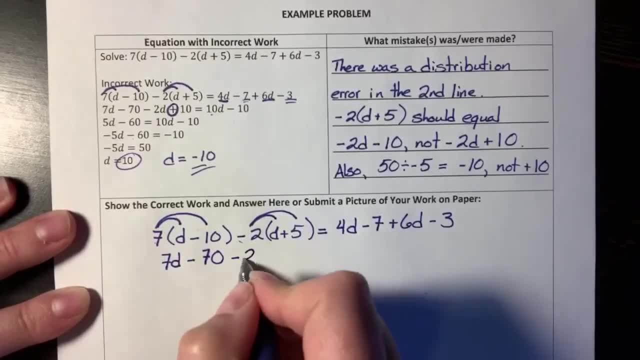 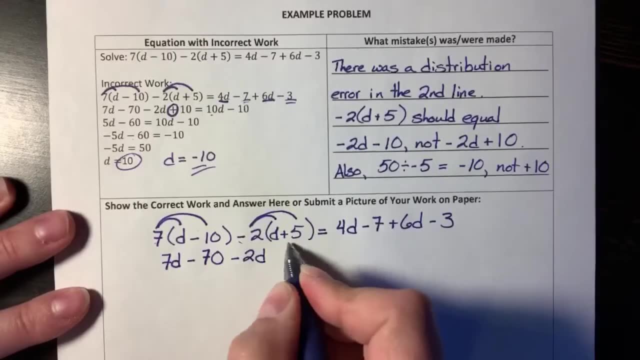 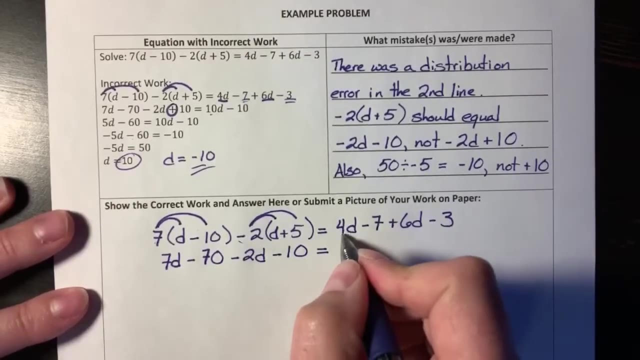 Negative two times D is negative two D. And then here was the mistake from before. We're not going to make that mistake. Negative two times positive five is negative 10.. On the right side I see some like terms, So let's go ahead and combine those together. 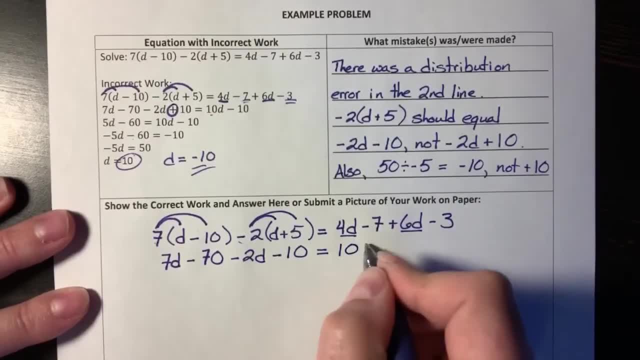 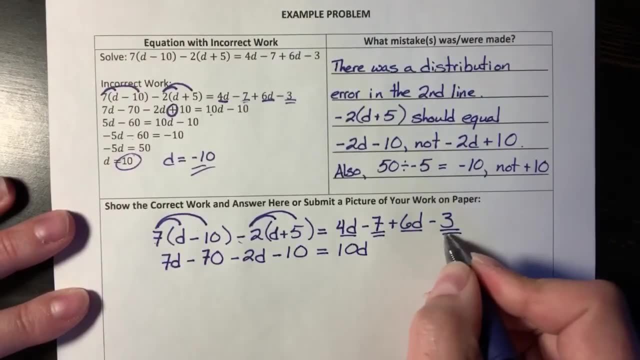 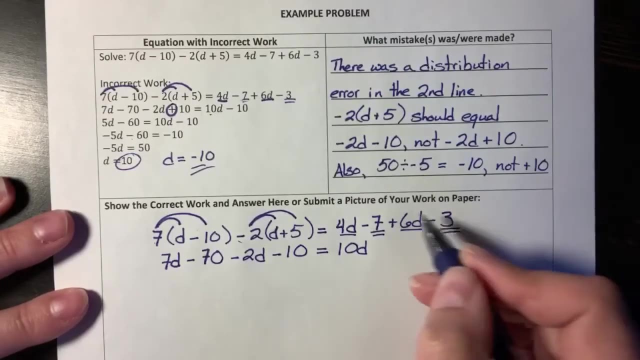 Four D and six D make 10 Ds And then I have negative seven and negative three, Negative seven and a negative three. You can do this on your calculator Or keep in mind that if they have the same sign, you're basically adding the numbers together but keeping that sign. 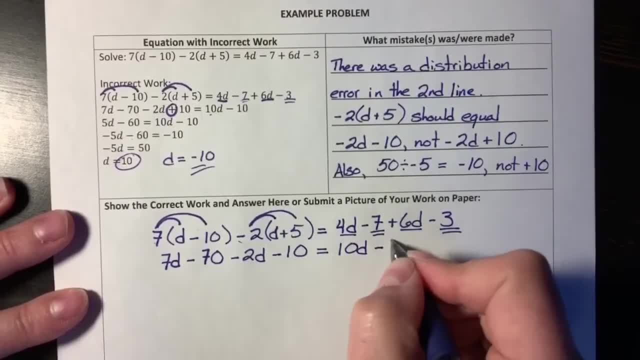 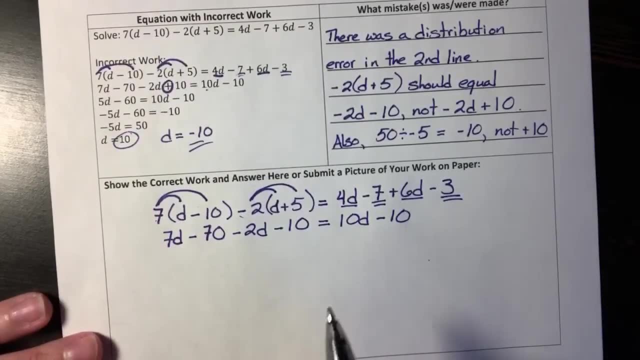 So it's definitely going to stay negative. And seven and three make 10.. So now we have our new second line. We're going to keep going here On the left side. let's see if I can simplify that a little bit. 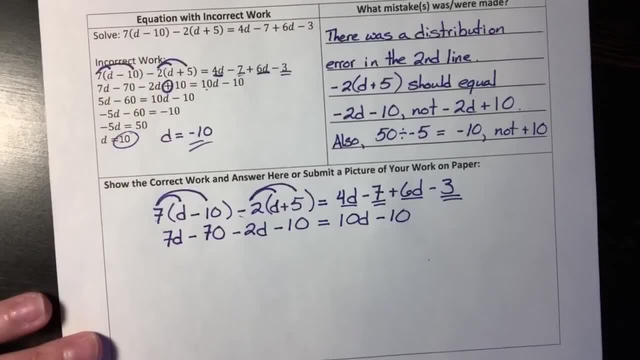 Because right now I have one, two, three, four terms in there And that's a lot. So let's see if I can combine some like terms. I see seven D and I see a minus two D over there, So those are like terms. 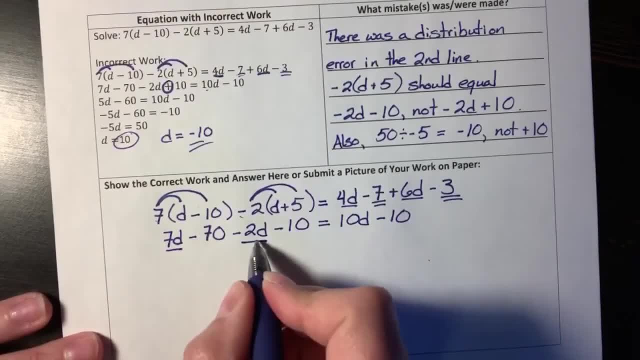 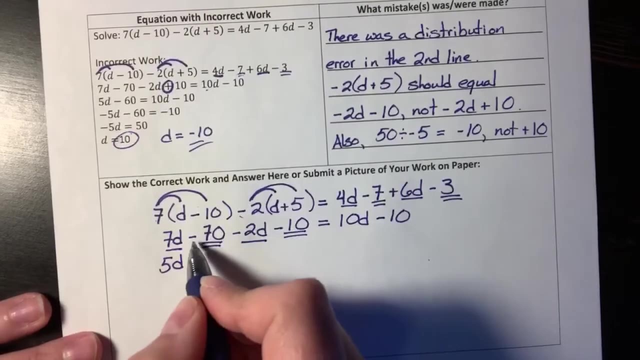 I'm going to go ahead and combine those: Seven D minus two D is five D, And then I have these two constant terms, which just means that they don't have a variable attached to them, They don't have a letter. I have negative seven D and a negative 10.. 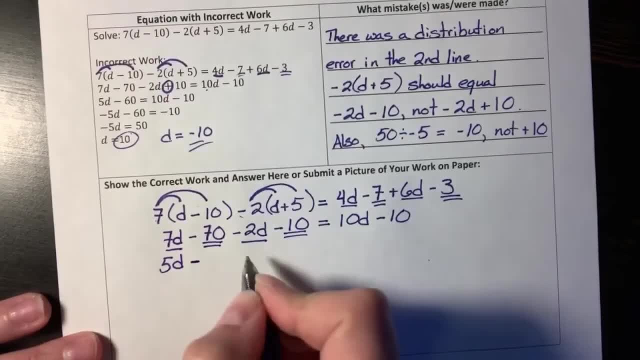 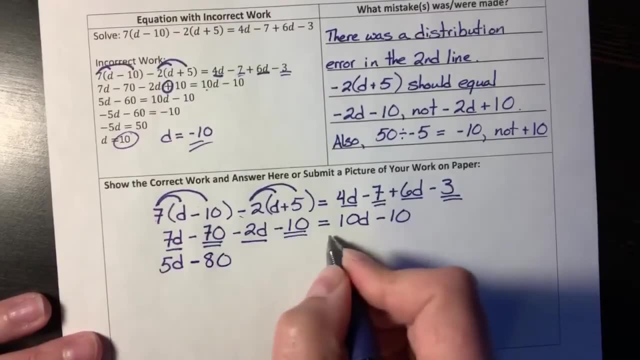 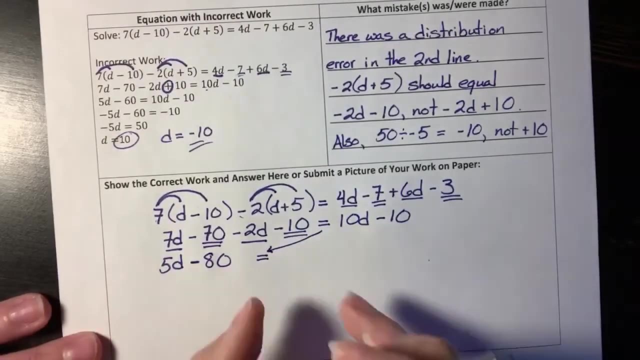 Same sign. So I'm going to keep the negative 70 and 10 make 80. And that's it for the left side. I still have my equal sign. So I'm just going to kind of scoot it over here, You know, kind of just move it over, just so I'm not having a big blank space between. 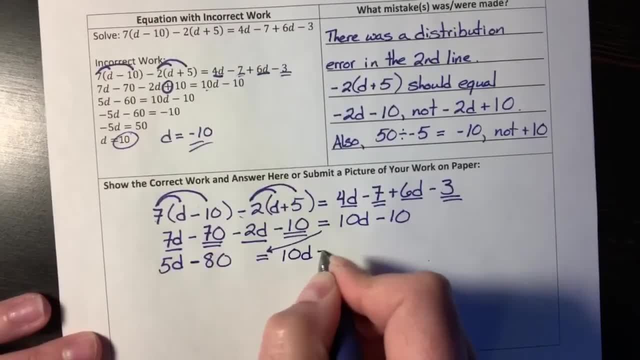 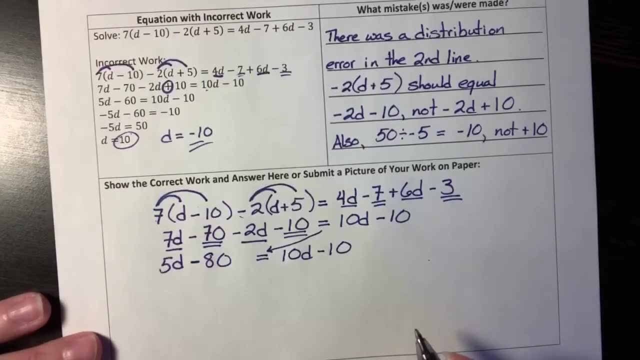 And then I'm not going to do anything to the right side right now, I'm just going to keep the negative, or 10 D minus 10, the same. Now you could take a little bit of a detour from how they solve the problem. 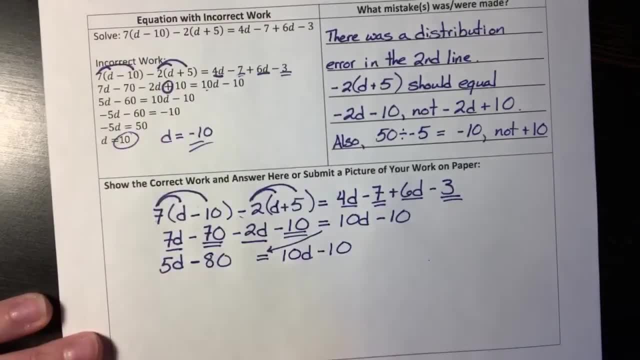 They had put the D's on the left side. Some people really, really like to keep their variables on the left side of an equation. You don't have to. You could move this five D over to the right side. So if you choose to do that, that's no problem. 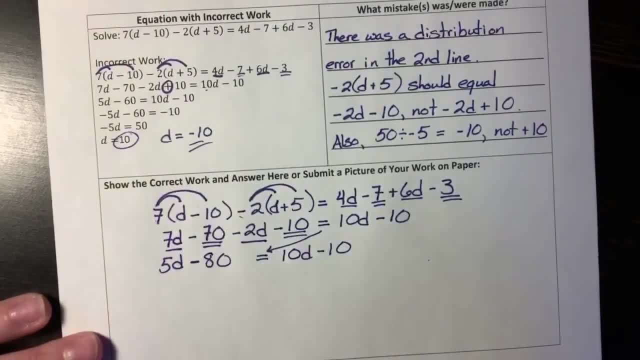 I'm just going to stay consistent with how the problem was solved earlier. Okay, So what I'm going to do now is I'm going to move this 10. D to the left side, because if I see 10 D and I want it to disappear from the right side. 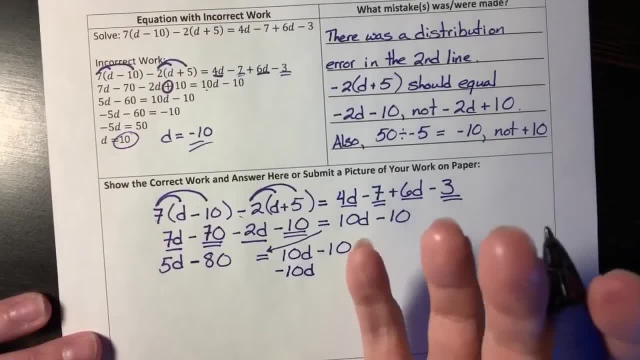 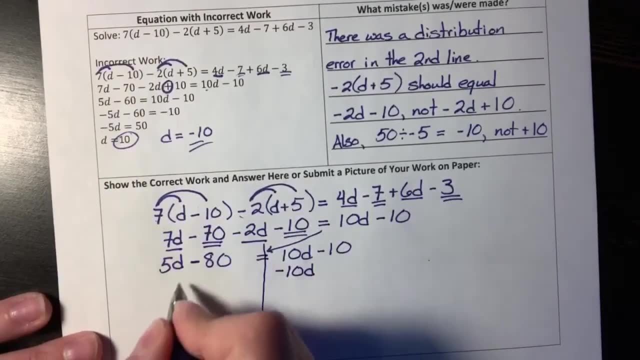 I'm just going to subtract it, I'm going to take it away And the rule is: whatever you do to one side of an equal sign due to the other, You can draw your line here if you want. So I'm going to do minus 10 D and draw my line, and five D minus 10 D. 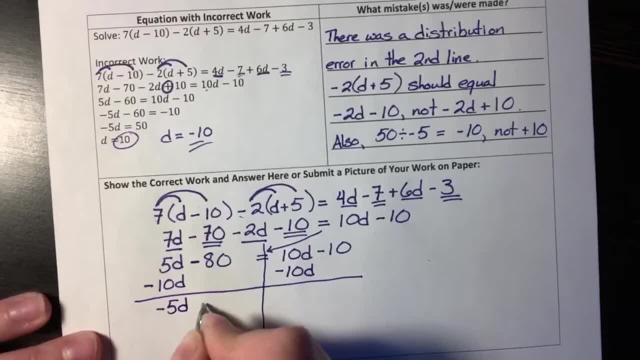 That is a negative five D. I'm going to bring down the minus 80.. I'm going to keep my equal sign And on the right side, this 10 D minus 10 D. Those are going to cancel and I'm going to be left with negative 10.. 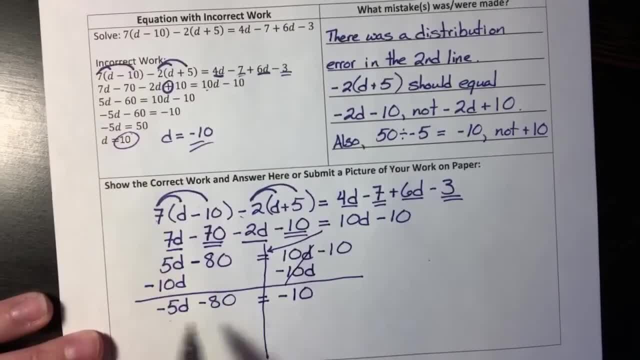 Now I'm still trying to get D by itself on the left side. So I'm going to go ahead and I'm going to do the opposite of what I see here. I see subtraction of 80. So I'm going to add 80 to both sides. 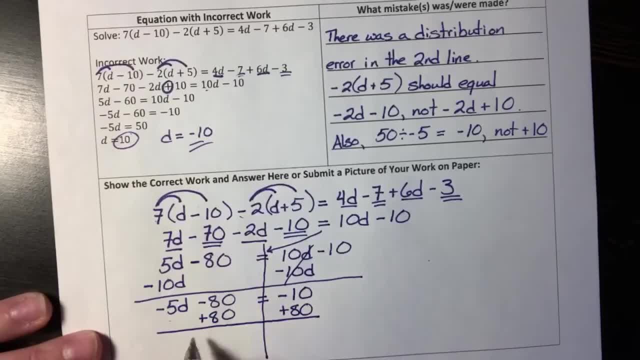 Draw my line on the left. Now these two cancel, So I'm left with just negative five D on the right side. Negative 10 and 80 makes 70.. Very different answer from before. Previously we had negative five D equals 50.. 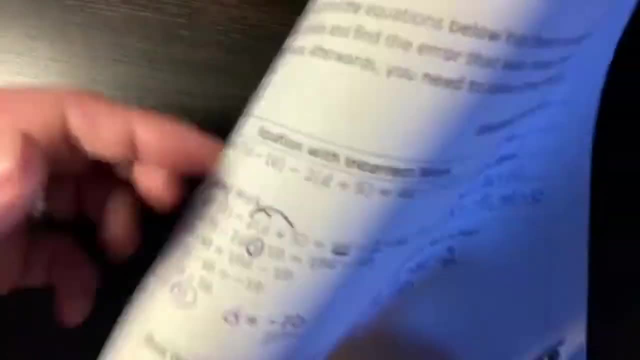 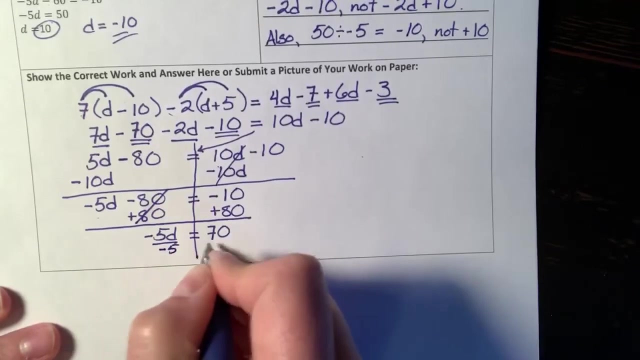 Now I have negative five D equals 70, because we didn't make the mistake, The person from before- And my last step here is going to be to divide both sides by negative five, Because if I see negative five D, that's multiplication. 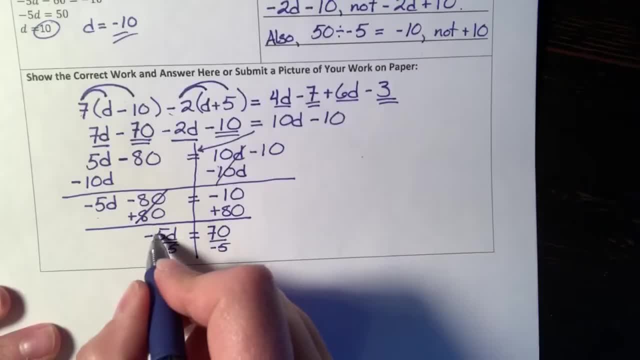 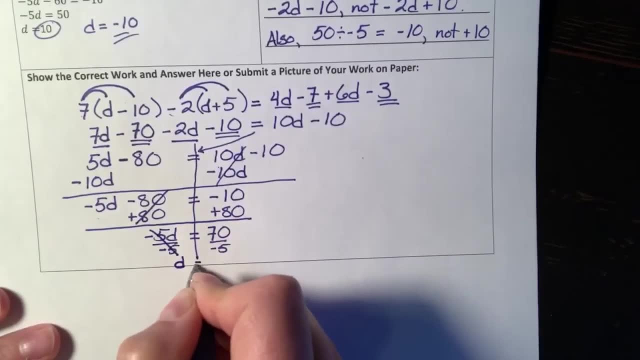 To undo multiplication. you divide Negative five divided by a negative five is going to cancel. Turns into a one, technically, A one D. I'm going to keep my equal sign. And 70 divided by negative five, That's going to end up being a negative answer. 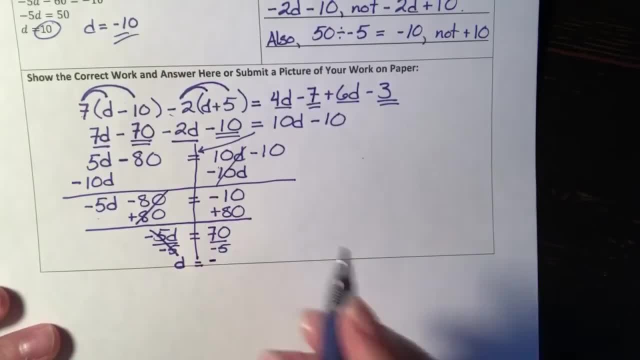 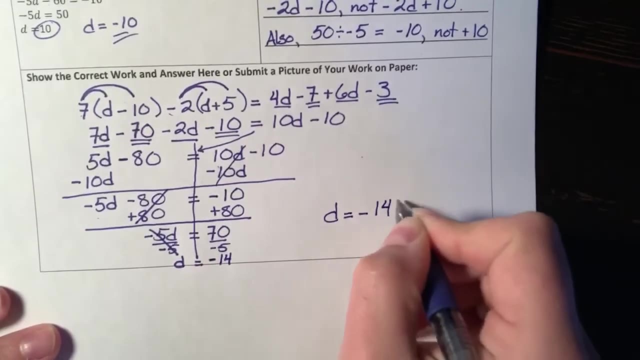 Because positive divided by negative five Is negative 70 divided by five. You can either do this in your head or use calculator, But you should end up with 14.. So our final answer Should be: D equals negative 14.. And there you go. 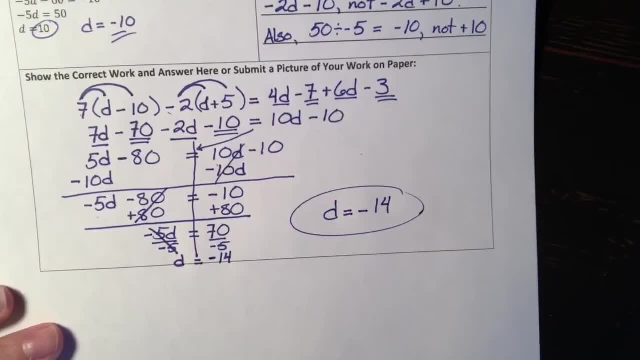 That's how you're going to be doing these error analysis Review questions.